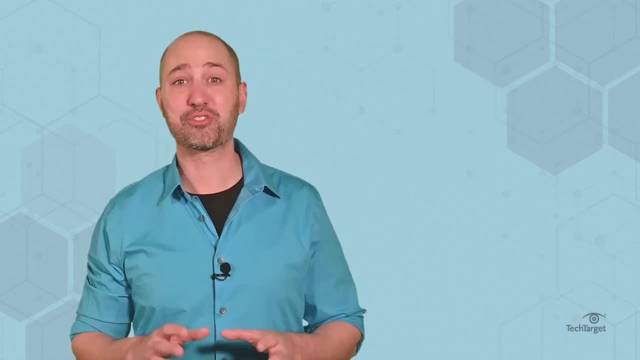 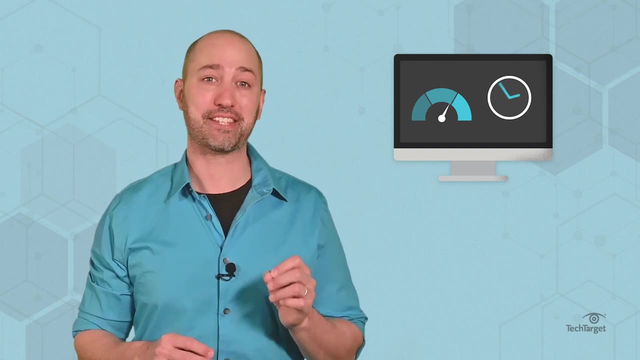 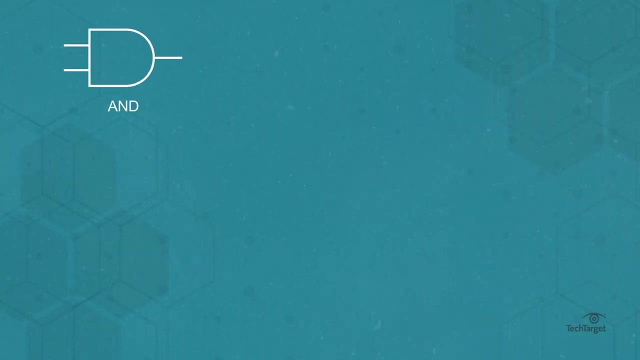 tablets and memory devices. Combining tens, thousands or millions of logic gates makes it possible for a computer to perform highly complex operations and tasks at ever-increasing speeds. There are seven basic logic gates, represented by specific symbols AND OR. 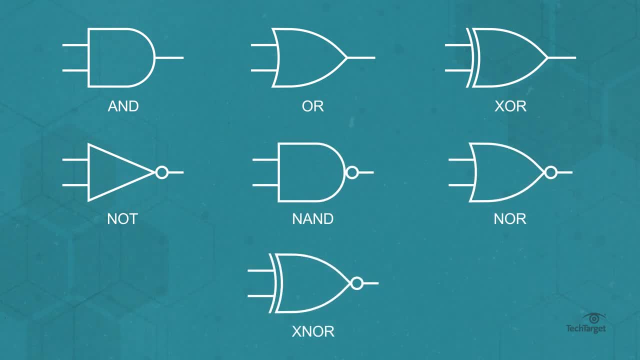 XOR, NOT NAND. NOR and XNOR, Two common types of flash memory, NOR and NAND flash, are named for the logic gate architecture they resemble, which you can read more about by clicking the link above or in the description below. 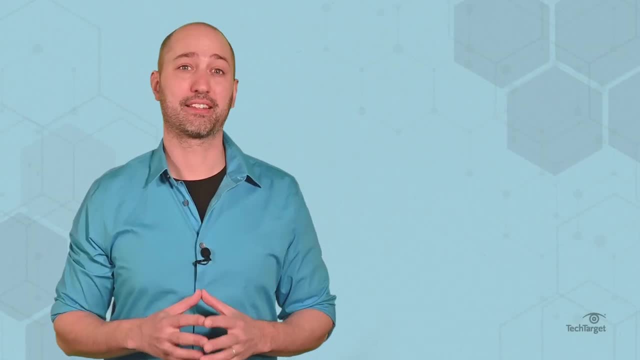 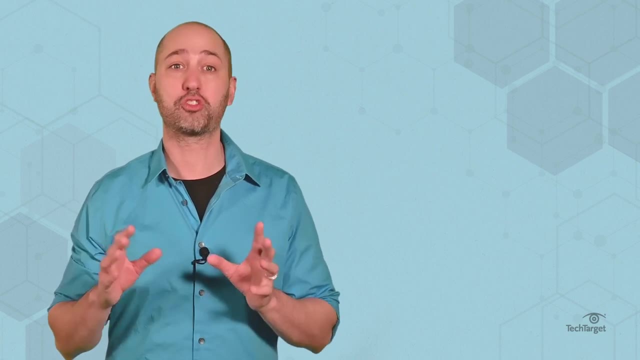 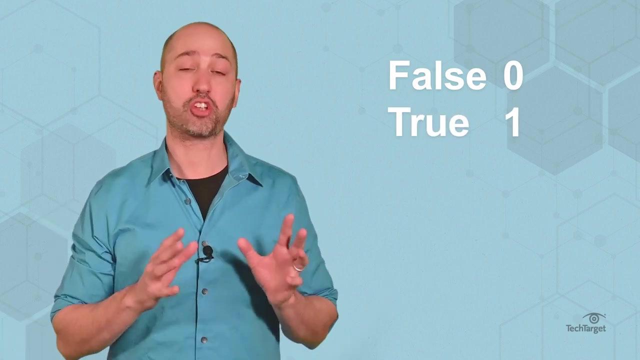 So what is a logic gate? Think of a logic gate like your light switch: It's either in an on or off position. Similarly, the input-output terminals are always in one of two binary conditions: False or zero, and true or one. Each gate has its own logic or set of rules. 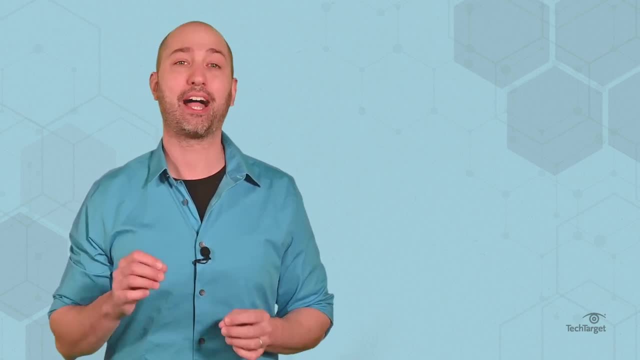 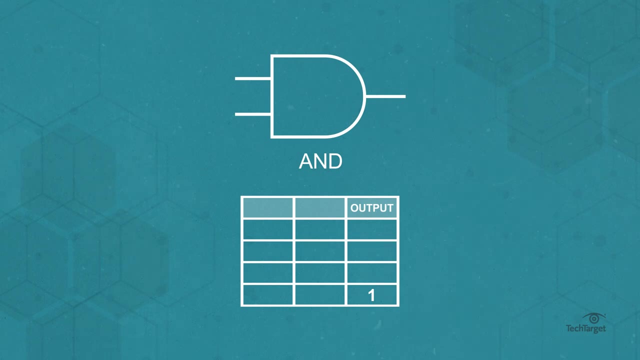 that determine how it acts based on multiple inputs outlined in a truth tip. For instance, the AND gate is named as such because the output is one only when both input 1 and input 2 are true or 1.. If only one input is true and the other is false, the output will be. 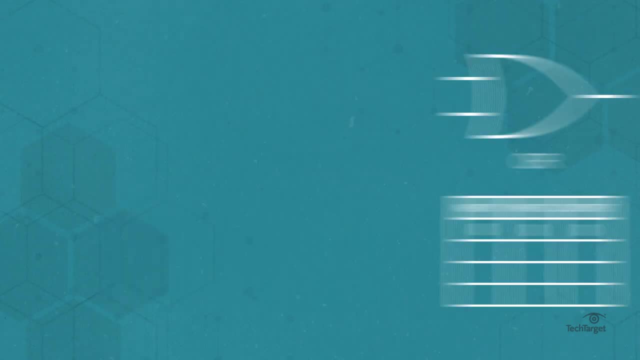 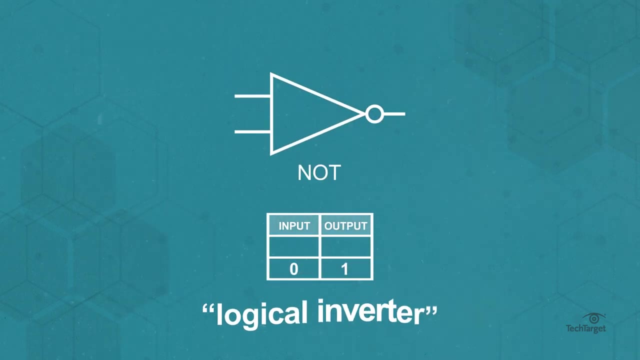 true or zero. Using this reasoning, the OR gate has a true output if one OR both inputs are true. The NOT gate is also known as a logical inverter. This gate only has one input and reverses the logic state. so if the input is 1, the output is 0. 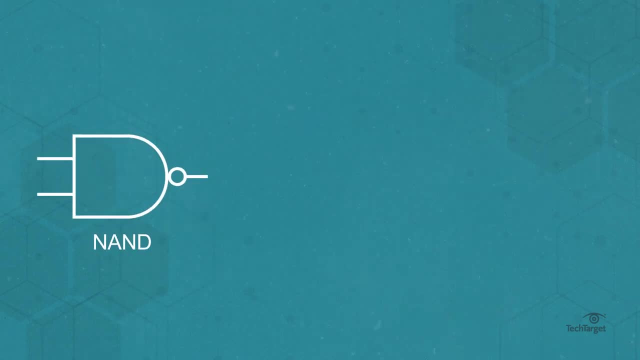 if the input is one, the output is zero. NAND, NOR and XNOR are inverts of their respective gates. So, for example, a NAND gate is an AND gate, followed by a NOT gate. If both inputs are true, the output is false. In theory, there's no limit to the. 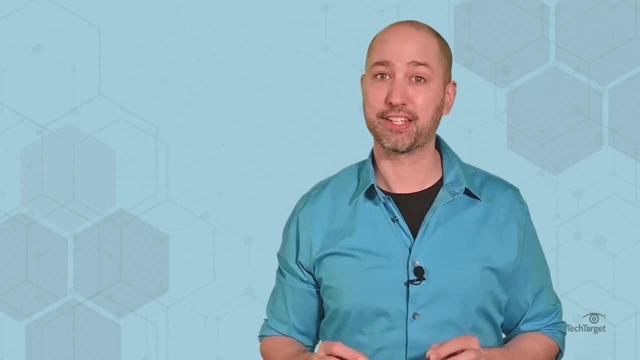 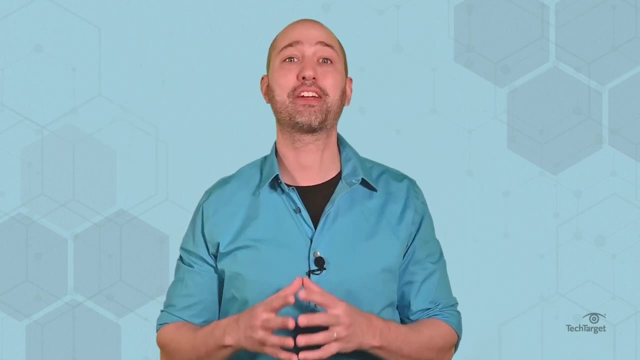 number of gates that can be arrayed on a single device, But in practice only a certain amount can be packed into a given physical space. What questions do you have about logic gates and their role as integrated circuit technology advances? Drop them in the comments below, and be sure to hit that like button.